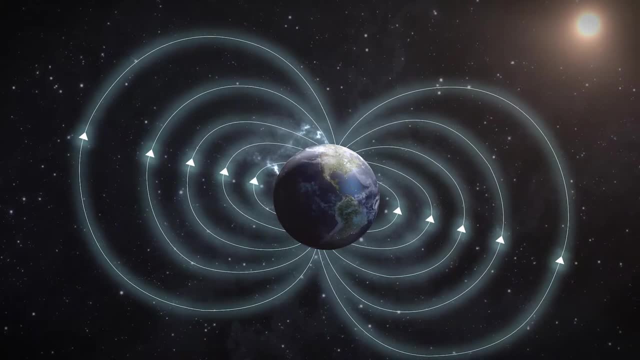 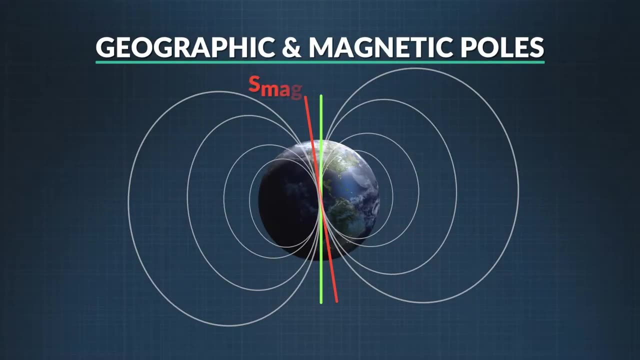 own magnetic field, which looks like this: See how the fields are concentrated at the north and south poles. Now here's a tricky thing to remember. The magnetic south pole is actually near the geographic north pole, And the magnetic north pole is near the geographic south pole. Scientists realized that opposite. 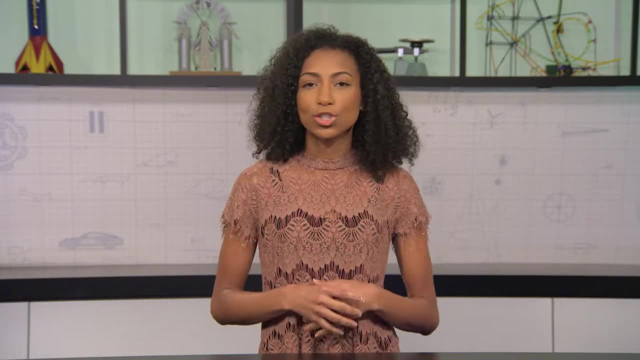 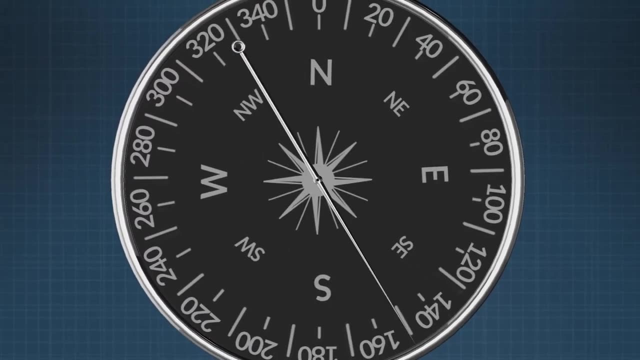 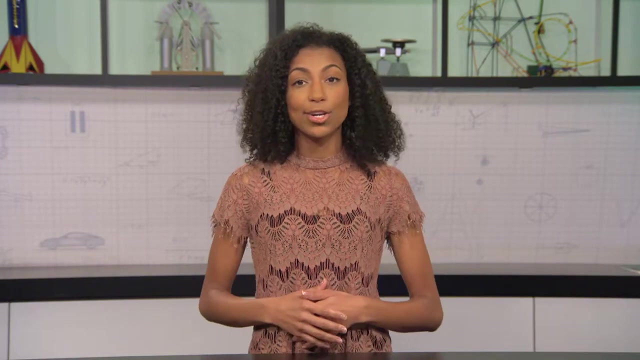 magnetic poles attract and light poles repel, just like electric charges. They decided this was a more accurate way to talk about magnetic poles. So when a compass needle spins, the north end is drawn to align with Earth's magnetic field. By the 17th century people had observed that electricity could create magnetism and vice. 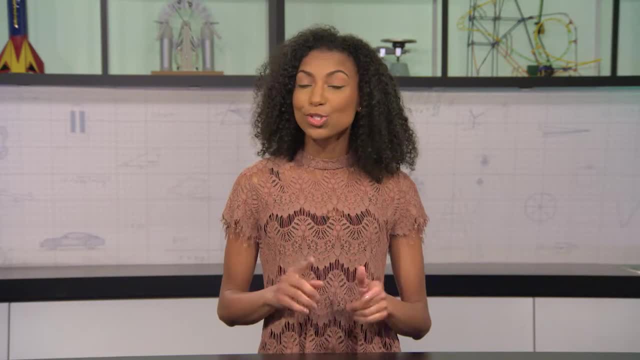 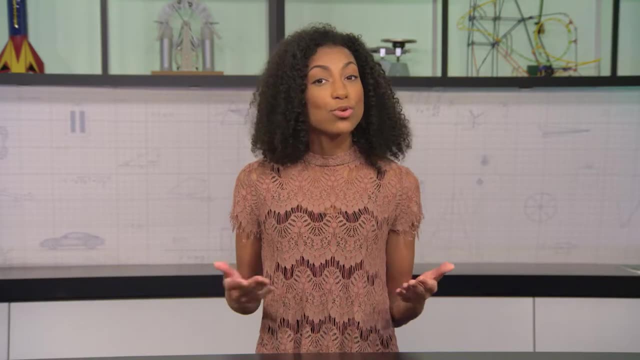 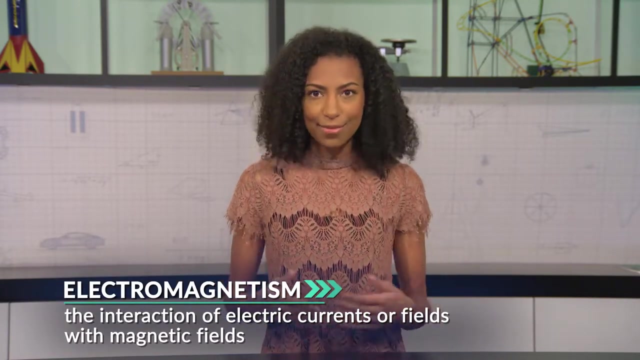 versa, Magnets can generate electricity. But then, about 200 years ago, a group of scientists, a guy named James Clerk Maxwell, nailed it when he realized that electricity and magnetism are two aspects of the same force: the interaction of electric currents or fields with magnetic fields. It's an 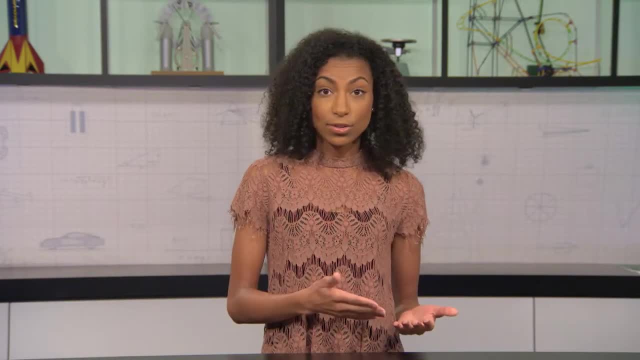 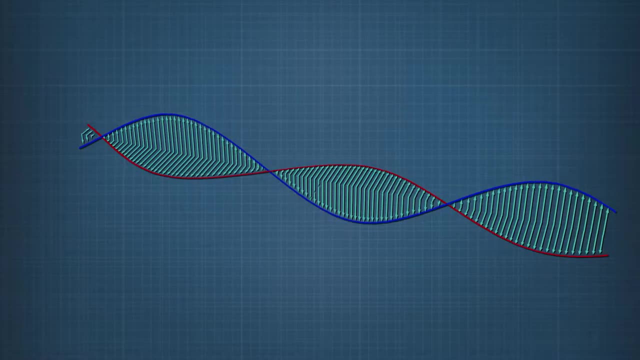 alternating kind of effect: Electricity creates a magnetic field which can generate electricity, and so on. You can see how closely they are related in this animation of a ray of light. Electricity and magnetism both arise from the interaction of electric currents. The magnetic field is 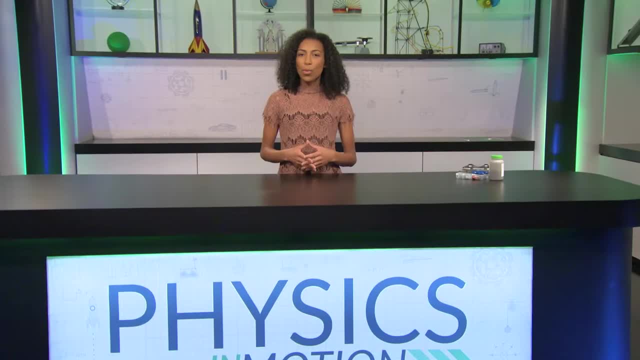 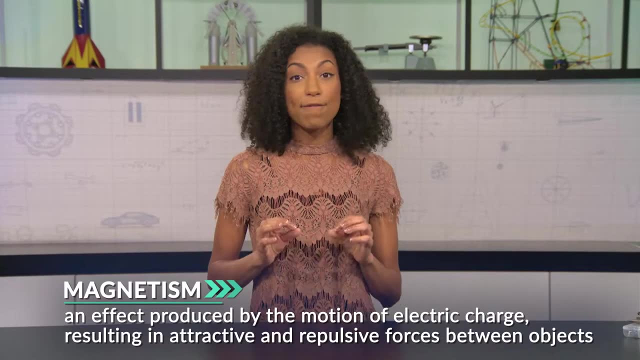 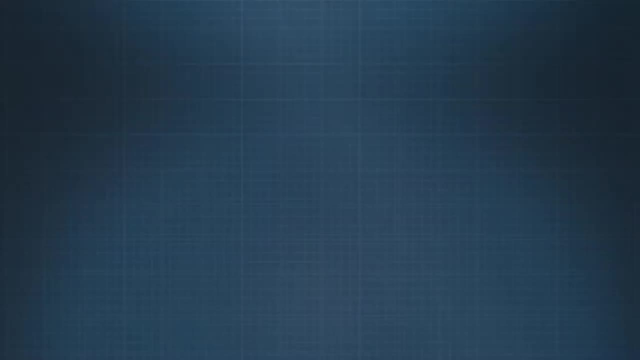 a magnetic field and the particles are electrically charged particles. We've talked a lot about what electricity is in earlier segments in this unit, But what exactly is magnetism? We can define it as an effect produced by the motion of electric charges, resulting in attractive and repulsive forces between objects. It's different from. 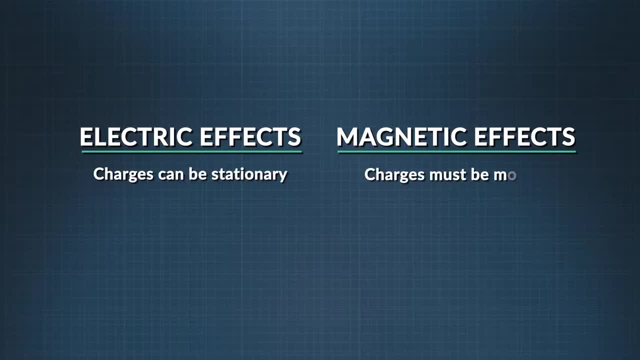 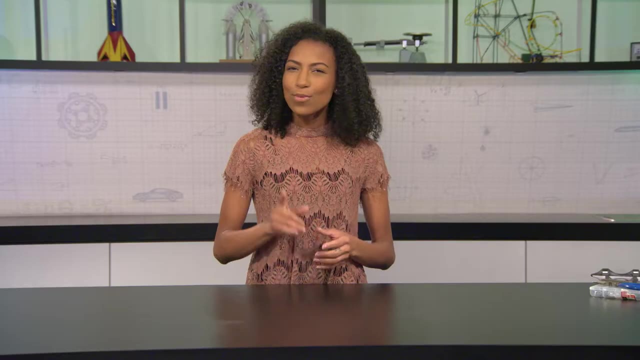 electricity in a couple of ways. One is that a magnetic field occurs only when charges are moving, but electric fields are created whether the particles are moving or not. Second, magnetic poles are always produced in pairs, whereas electric charges are not. Now, one cool thing about a magnetic force is that it can act at a distance. Let me do. 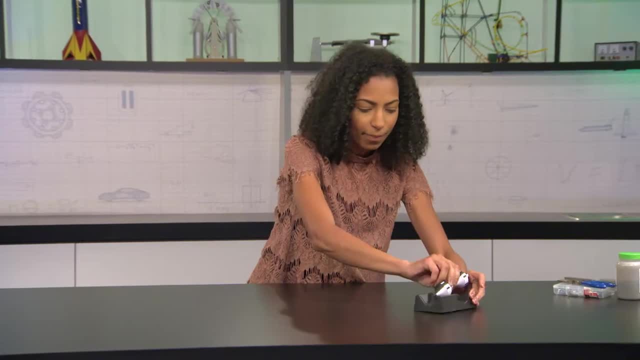 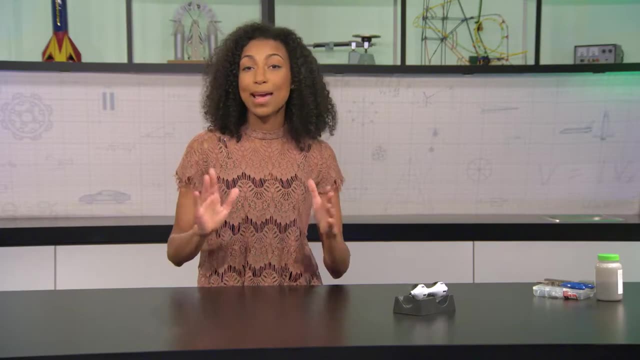 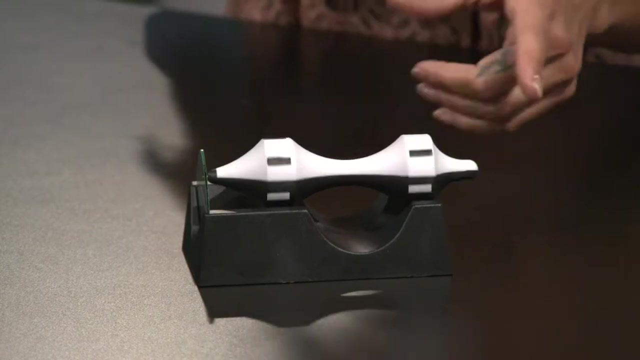 a little magic trick. You see how it looks like it's levitating. Well, in fact it is levitating courtesy of the magnetic field. How does it work? This end of the magnet is north. You usually call the magnets north pole, And this one is north too. 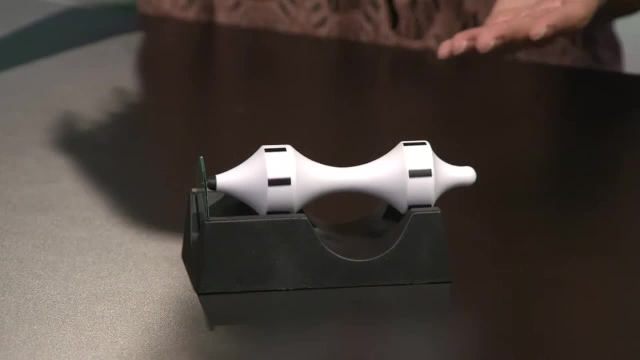 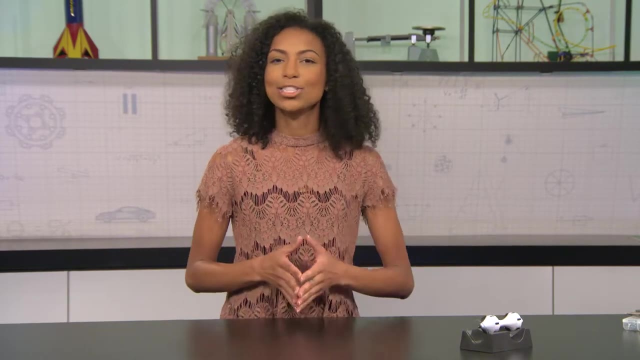 So what do you think happens? The light poles repel each other, keeping the magnets apart. They don't have to touch each other to affect each other. The force is between them. Kind of like magic, isn't it? But it's science. 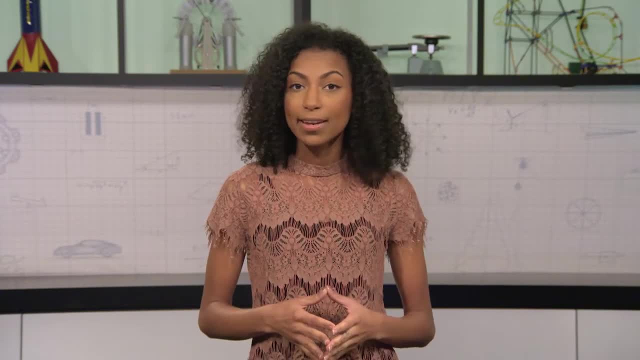 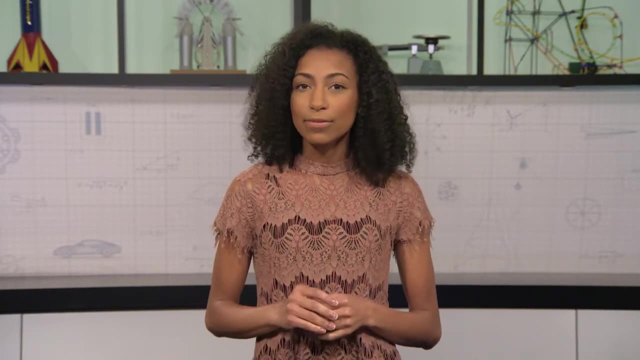 All magnets are miniature versions of the Earth, Like our planet. they have two poles, they create a magnetic field and they are affected by other magnets At the subatomic level. the electrons spin like tops, as well as spinning around the nucleus, creating magnetic. 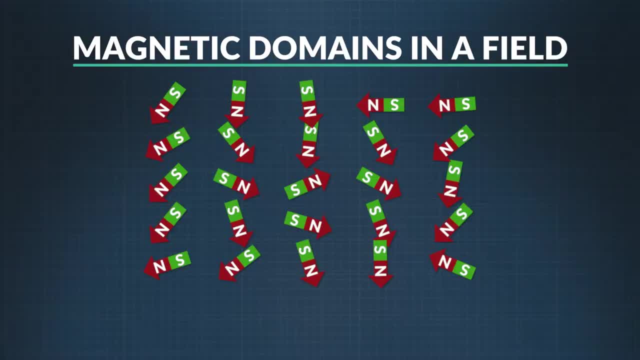 fields Within any piece of magnetic material are domains, areas where the individual magnetic orientations of atoms are aligned with one another, so they point in the same direction. Each of the domains also has a north and south pole. When the domains line up, that creates. 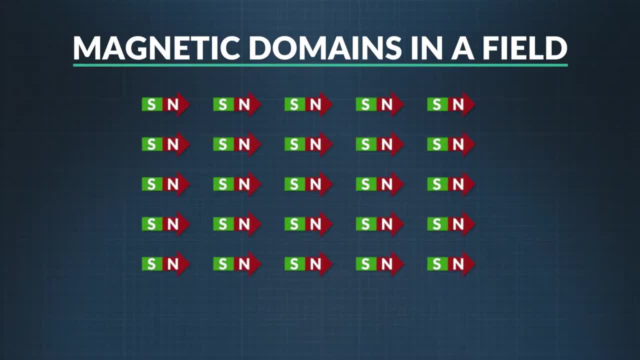 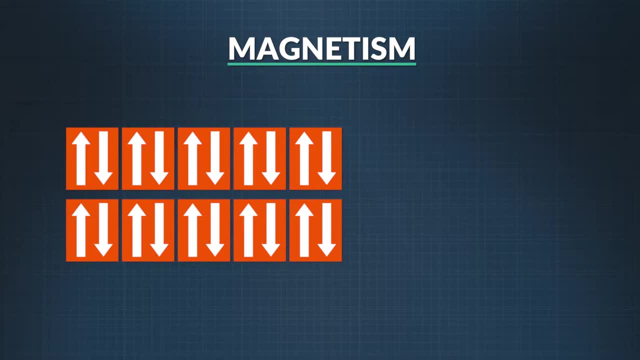 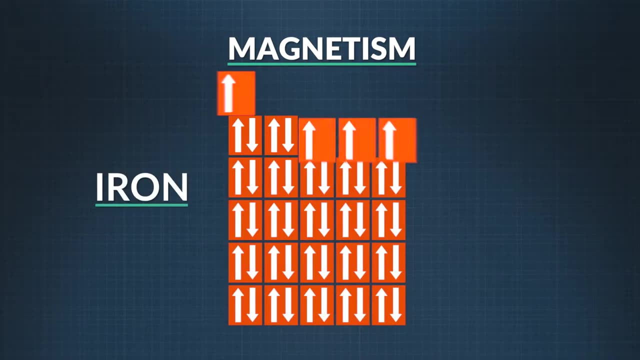 a magnet. So why isn't everything magnetic? Most electrons in an atom exist in pairs that spin in opposite directions, so the magnetic effect of one electron in a pair cancels out the effect of its partner. But if an atom has some unpaired electrons, these produce magnetic fields. 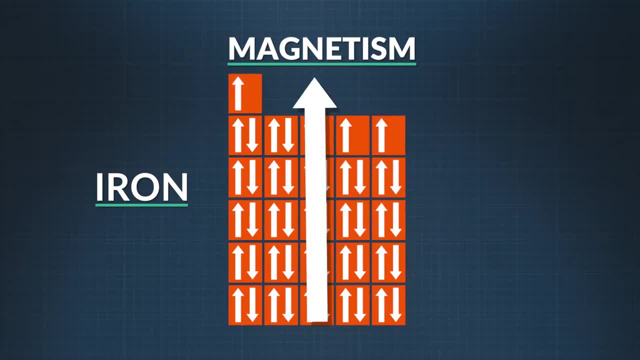 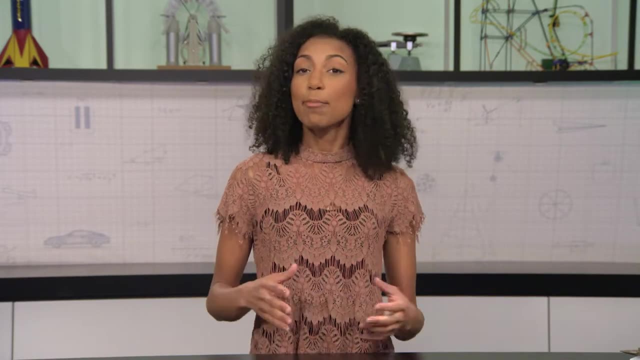 that line up with one another and turn the whole atom into a mini-magnet. In other words, when you put a material like iron, for instance, in a magnetic field, the electrons change their spin and align with the magnetic field. Now magnets can affect other materials in another way. They can make a temporary magnet. 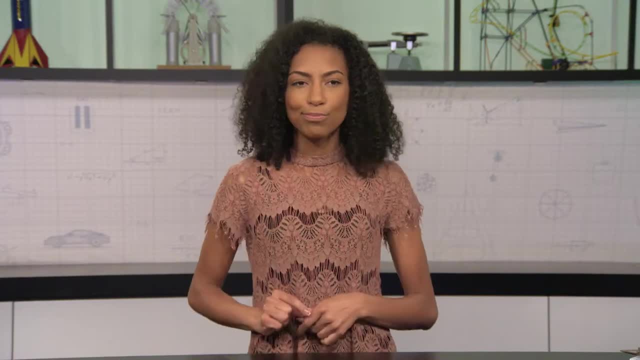 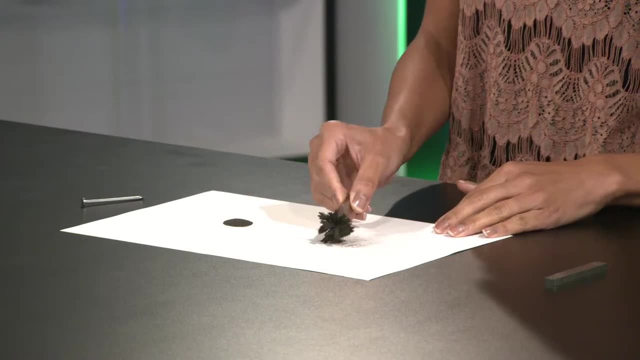 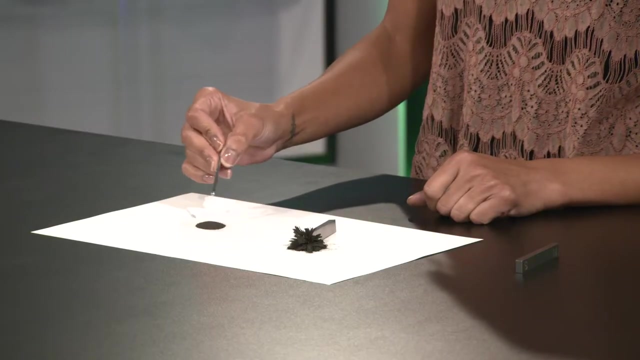 out of certain kinds of unmagnetized materials. Let me show you One magnet. Check See, It attracts these iron filings, One nail. But it's not a magnet. No attraction, See. Now I slide the nail with the magnet in the same direction, moving it away from the nail. 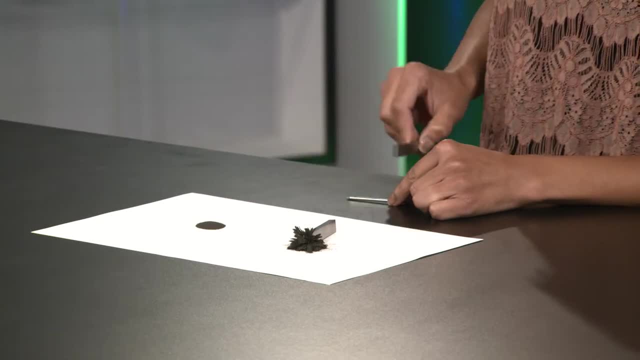 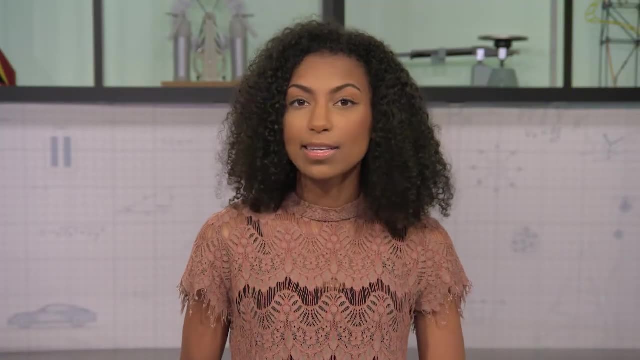 at the end of each pass. Each time I do this, more electrons in the nail align with the magnetic field. Now I've been aligning our domains for about 15 seconds. Let's see if we've got a magnet, and we do. 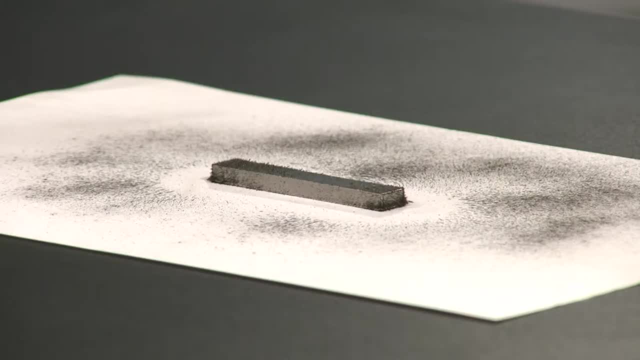 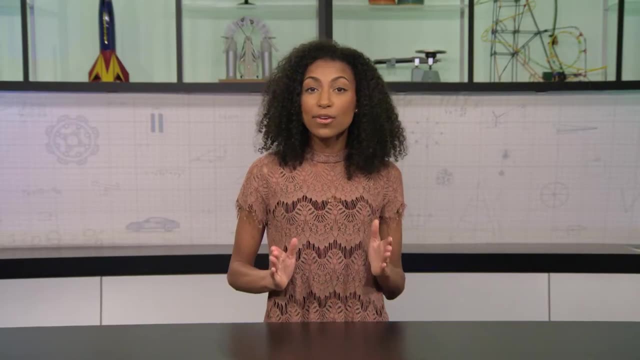 And let me show you something else. When I sprinkle iron filings on top of a bar magnet, look, You can see magnetic field lines. Like any force, magnetic force has a direction, such as up or down. If we want to know the 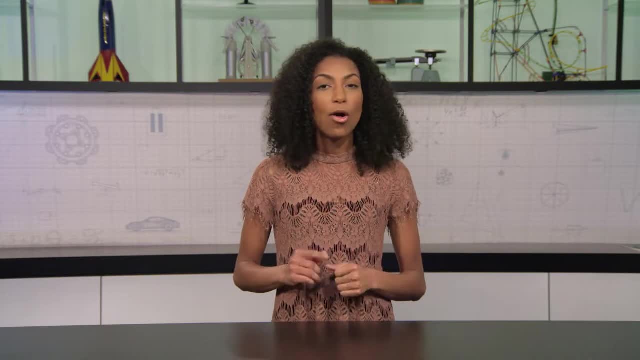 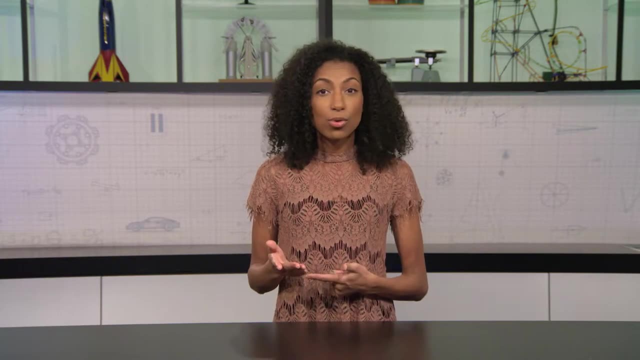 direction of the magnetic force. we can figure that out using what we call the right-hand rule. We know that the magnetic force acts only on charged particles. So let's see how the right hand rule works for a positive charge first. With my right hand, I make a thumbs up sign. 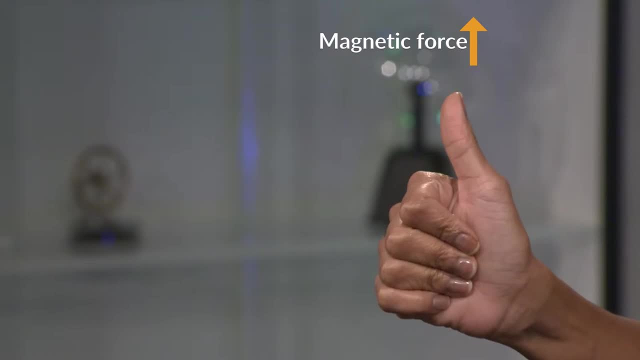 My thumb represents the direction of the magnetic force acting on a positive charge. Now I point my forefinger at a 90 degree angle with my thumb, My pointer finger represents the velocity vector of the positive charge, including the direction it is moving in. 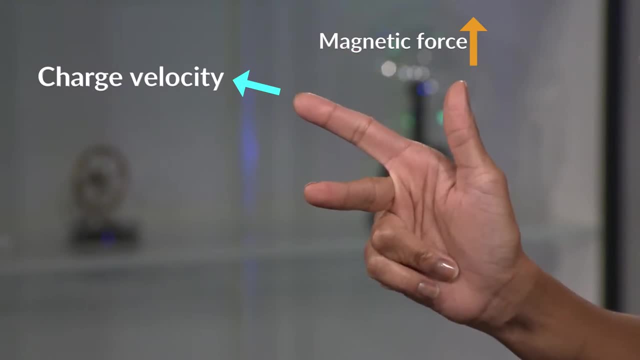 Then I take my middle finger and I point it at a 90 degree angle with my pointer finger. like this: My middle finger represents the direction of the magnetic field that the charge is moving through. If I have a negative charge, do the right hand rule the same way, but know that the 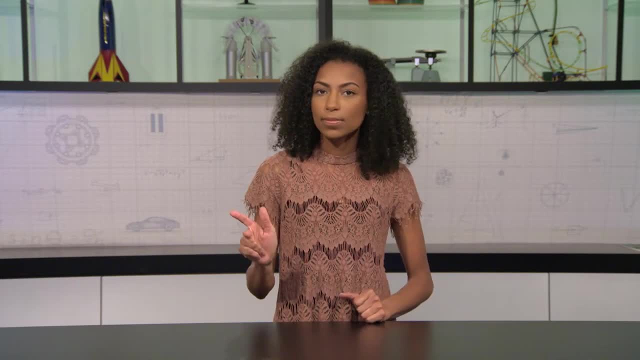 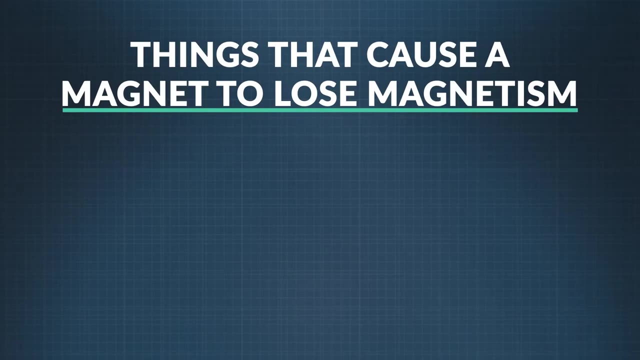 negative charge is in the opposite direction of the positive charge. If the positive charge is moving to the right, the negative charge would be moving to the left. There are three things that can cause a magnet to lose its magnetism. One is heating the magnet. 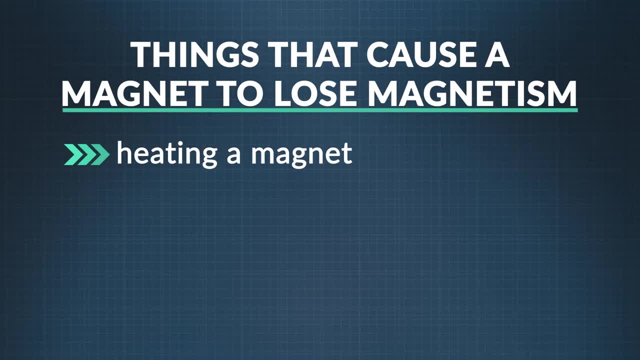 The heat makes the electrons move faster and faster, and as they get jumbled up, the magnetic force dissipates. Another is putting the magnet in a demagnetizing field, one that cancels out the magnet's strength. If you've ever had a magnetic strip on a card in your wallet, stop working. this may. 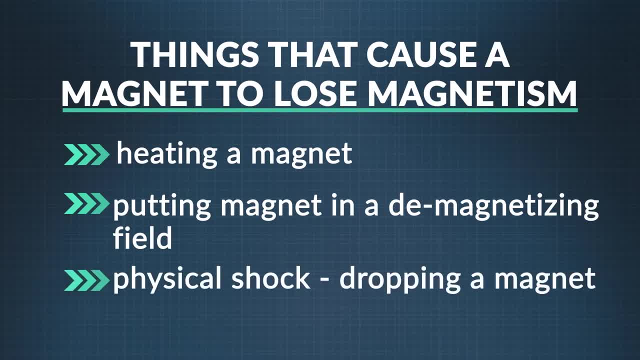 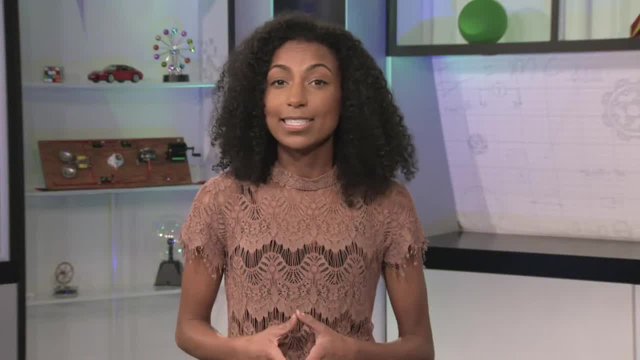 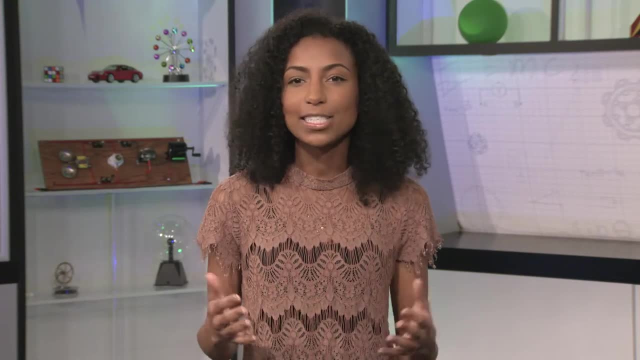 well be the cause. Finally, dropping a magnet will disrupt the alignment of its individual magnetic orientations and the magnetic force. So we've learned what magnetism is and how it behaves, how charge and motion creates a magnetic field, And remember that a charged particle has to be moving. 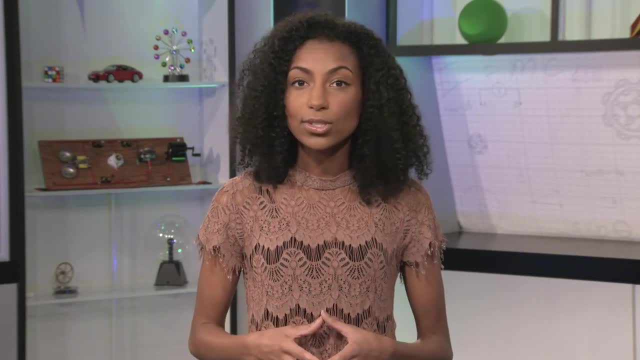 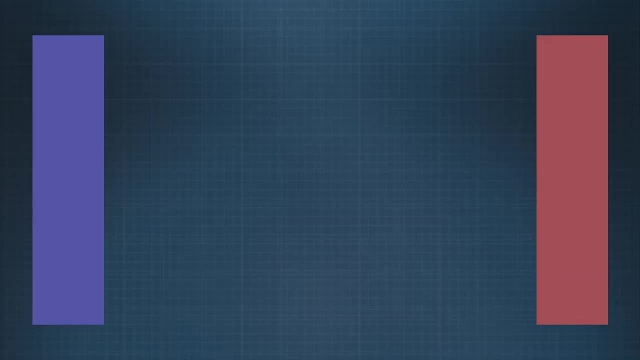 A magnet is moving through a magnetic field in order to experience a magnetic force. No movement, no force. Now let's look at how to calculate magnetic force. Let's say we have a magnetic field and there's an electron moving around in the field. 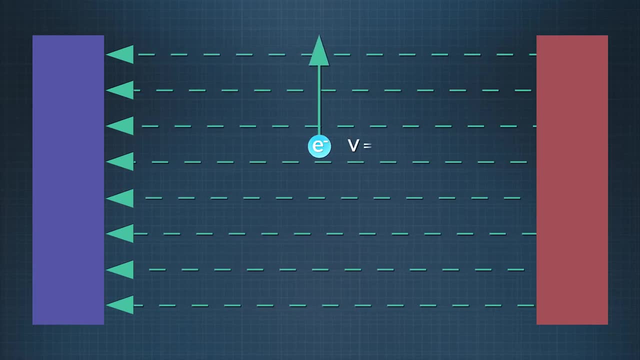 The electron is moving fast, at a velocity of 2 times 10 to the 5th meters per second upwards in a magnetic field strength for Teslas pointing from right to left. A Tesla measures the strength of a magnetic field. What will happen to that electron?